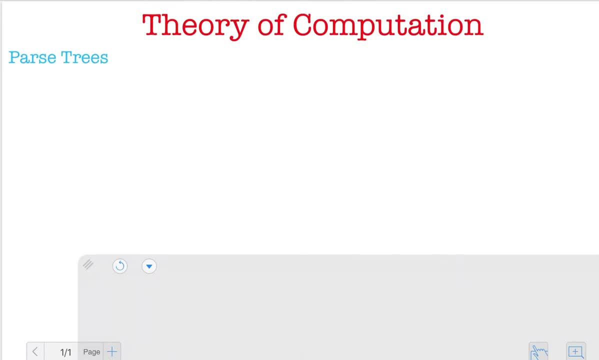 Hi everyone. so before we go to the other form that I was talking about for context-free grammars, there's some other things that I wanted to discuss, The first of which is parse trees. So we'll see what the parse tree is in a minute. 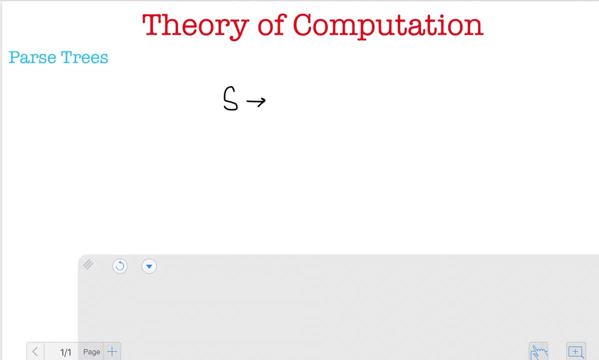 Let's consider a grammar. So let's say I have the grammar s goes to ss or a, and now I've been given a string. So the string that I've been given is, let's say, aaa. This is the string that I've been given and this is my grammar, right here. 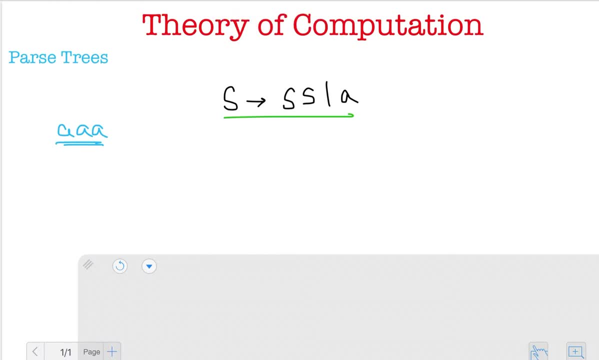 So I want to determine how this string was obtained from the grammar given. So I start with the start symbol, s, and that went to ss. and now one of these s went to again ss, So I got sss, followed by each of these s going to aas, So I'll get aaa. 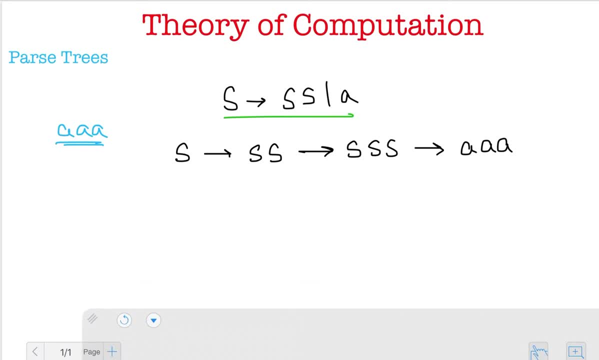 And what I can do here is I can draw a tree. So what I'm doing is I'm starting with s, I'm saying that that went to s and s, and at this point let's just assume that my left s is the one that split into 2s. So this one to s and s, and each of these. 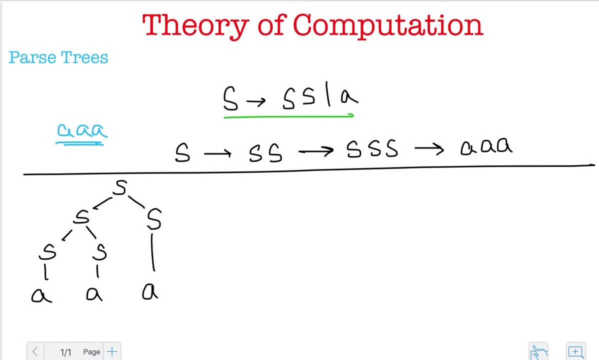 then went to a. So the string that I get at the bottom with my leaf notes is the string that I was given right here, And this thing that I've obtained is called a parse tree. So this is called a parse tree and that's basically so. I have now maybe wonder if I should have this Sekhat matin Doing a whole Cell. 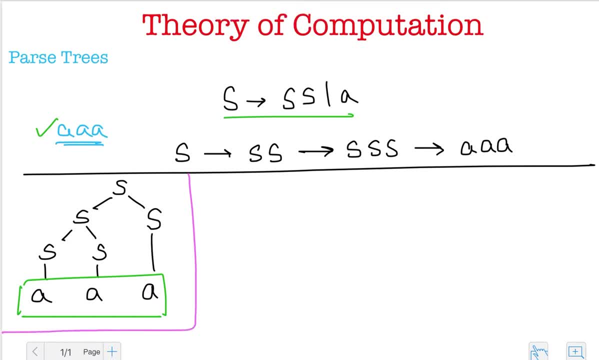 a passive material. I can, as I describe, I can express an object using a variable. For example, this is an object where, So it can be: aoui, maybe a lot, a lil bit, maybe, maybe, maybe, and that's basically what a pass-tree is. and one thing we want to remember is: 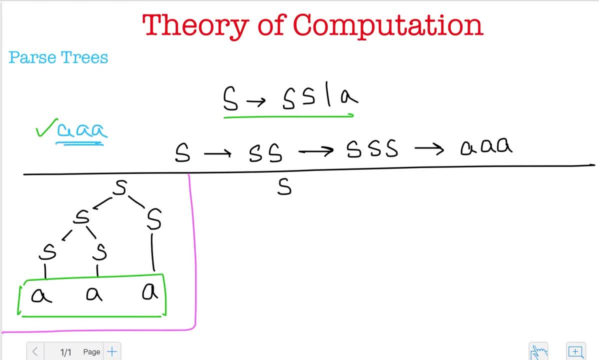 that there might be multiple pass-trees for the same string, so I could have this pass-tree for the same string that was given to me. so, as you can see, both of these give me the same string at the end, which is AAA, but these aren't identical.